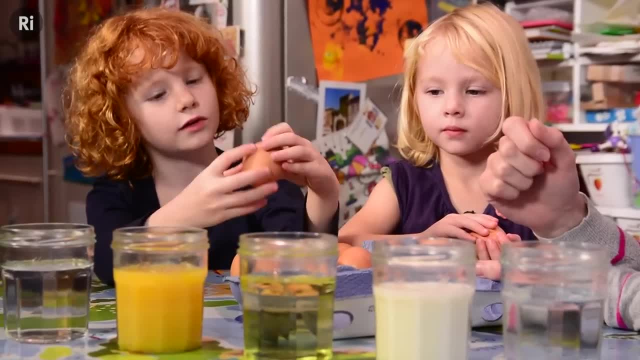 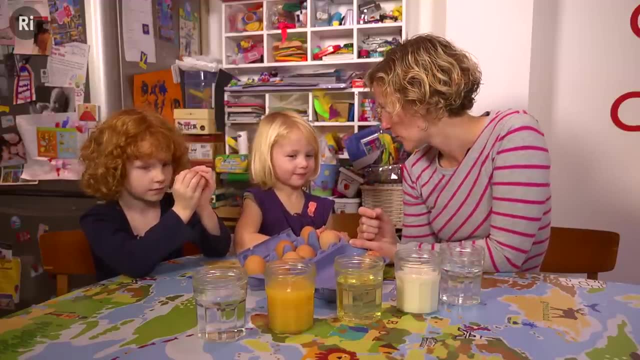 the same thing will happen to them in each of the jars. I think the same thing, Elodie. do you think anything different is going to happen in any of the jars? Which one, All, all In the oil? you think something different is going to happen? 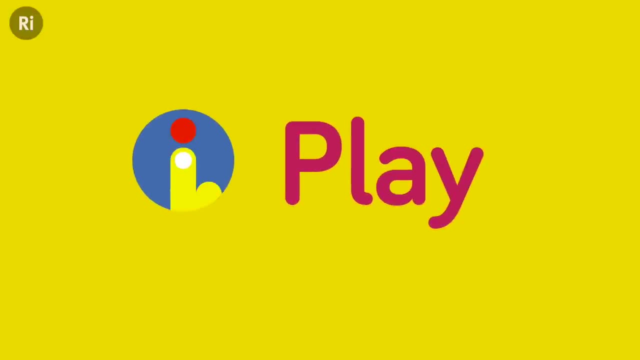 A little bit. You think something different is going to happen. Okay, cool, Let's put it in. You put your arms in the oil. Yum, good, Getting bigger. It does look bigger, doesn't it? Oh, hang on. 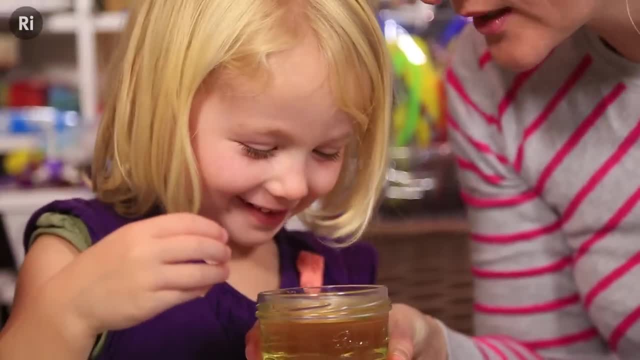 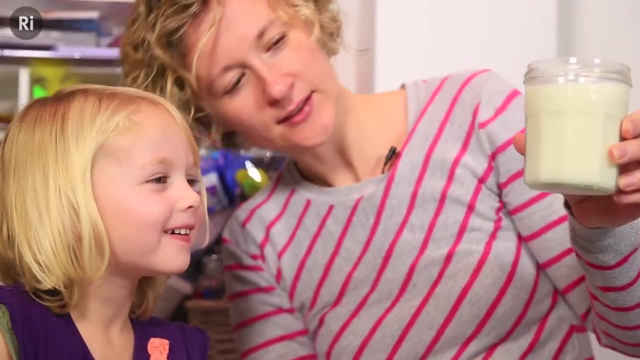 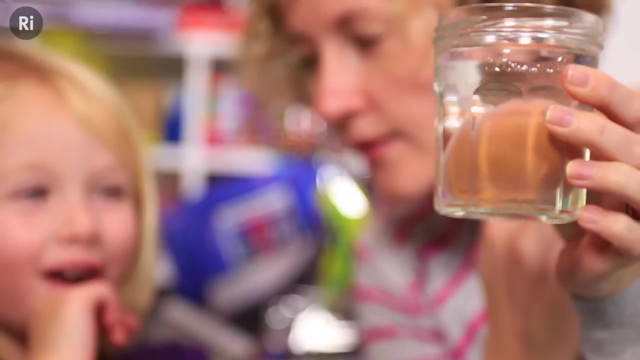 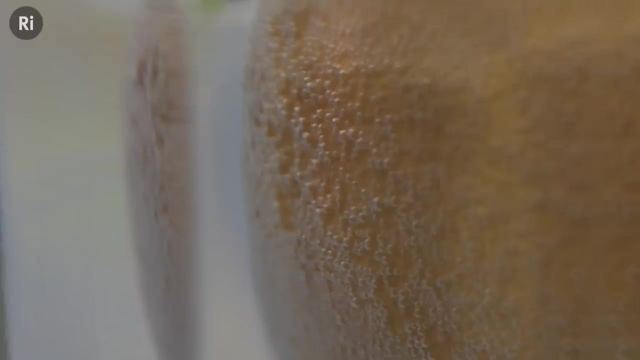 What's on the outside of the Turn it white? Yeah, little bubbles on the edge of the bottle. No, I think the outside looks better. The outside looks better, Yeah. Okay, so it's nearly lunchtime, so we're going to go away and leave these and see what happens. 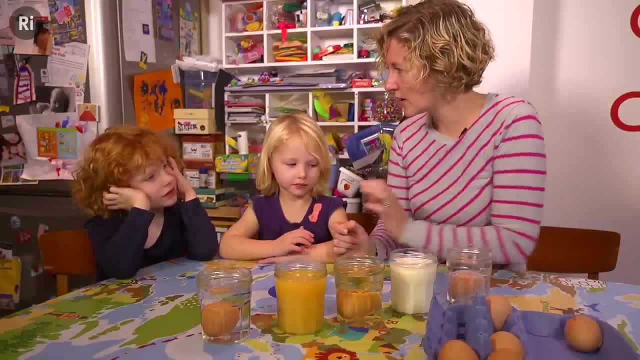 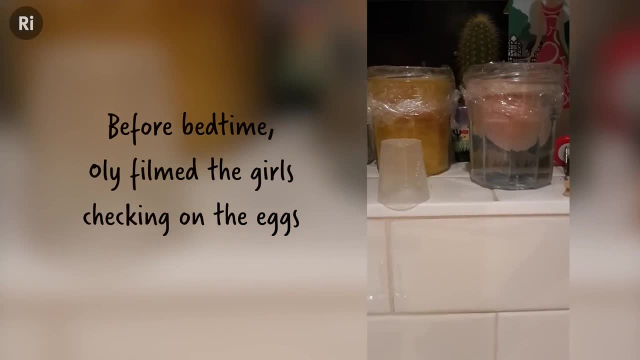 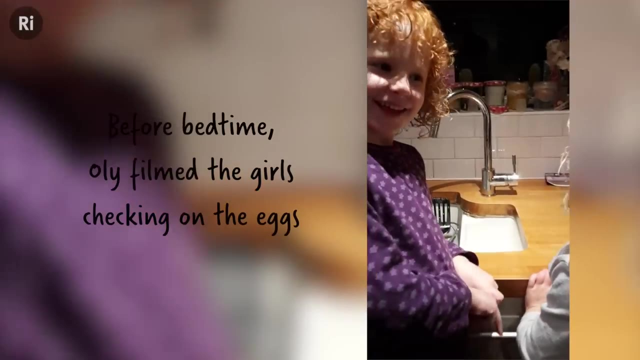 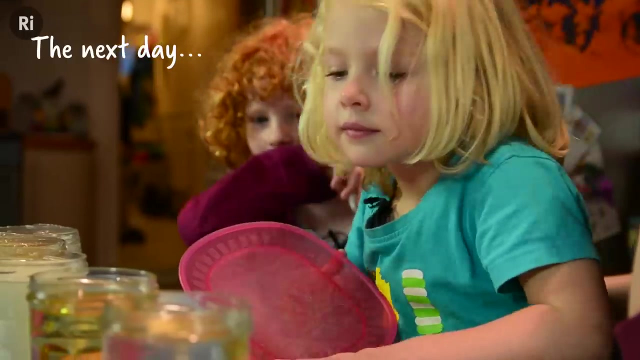 with the eggs in the vinegar and all of the other liquids and we'll come back and check on them later. Does it? Which one? The vinegar, because it's floating Night night eggs, Night night water, Night night things? Which ones have had something different happen to them? 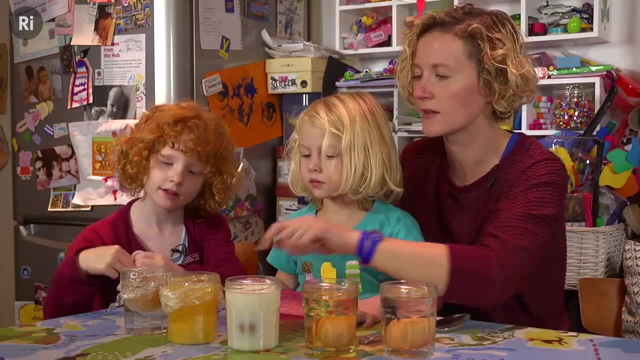 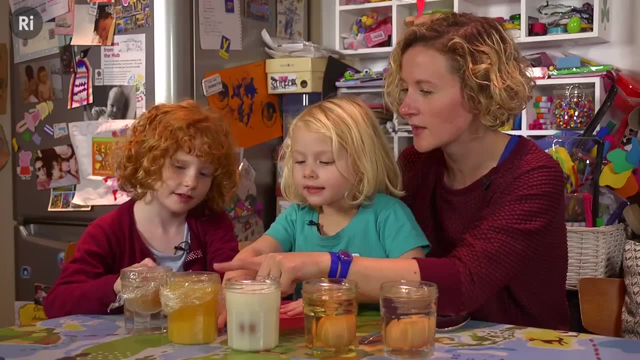 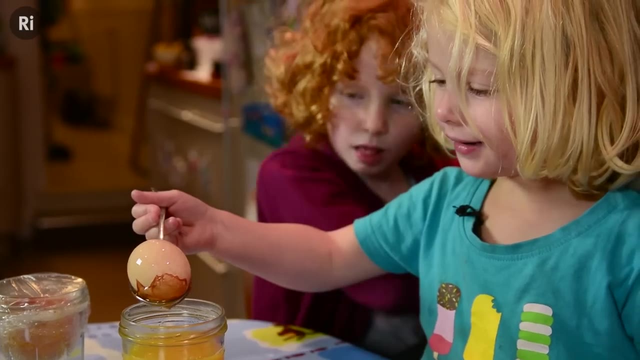 These two? And what were the eggs in here? A bit yucky. It does look a bit yucky, doesn't it? What's this one in though? Juice and vinegar. Investigating how different liquids affect an egg is a fun way to introduce children. 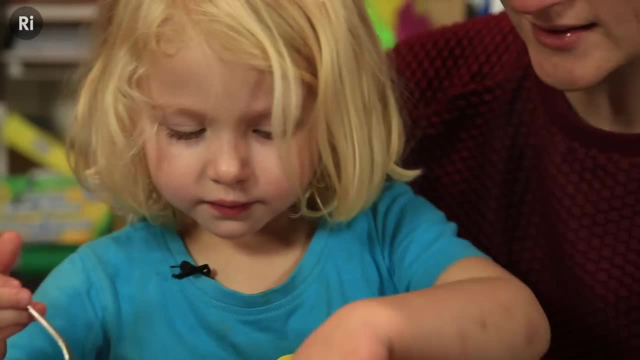 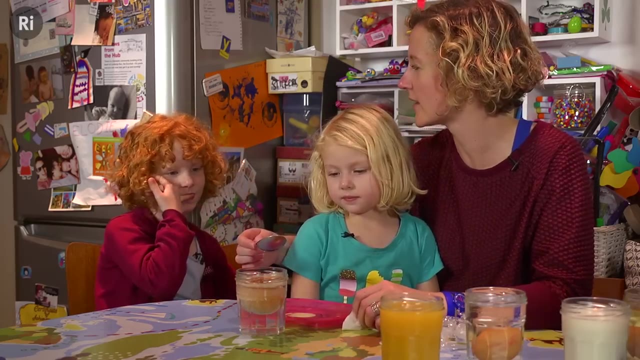 to the idea that different substances have different chemical properties, even though they might be the same in other ways. Who's going to be brave and take out this final egg? Do you feel brave? Elodie: No, No. Viola No. 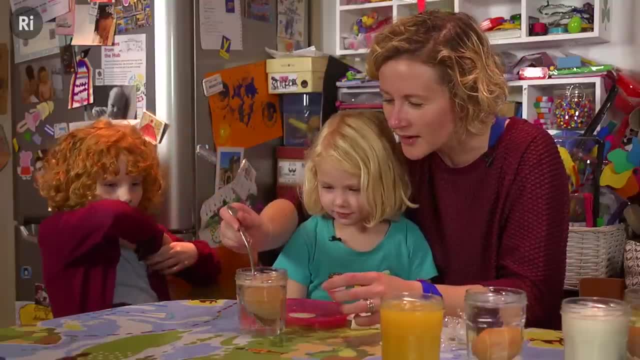 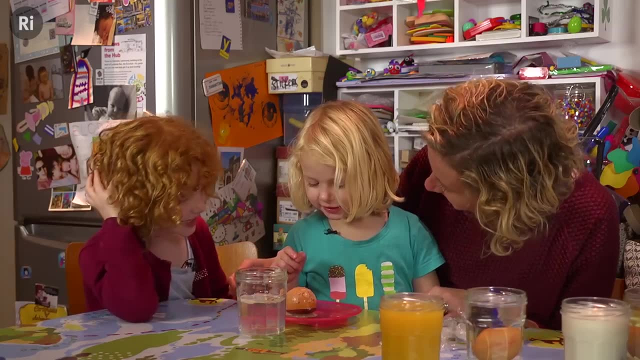 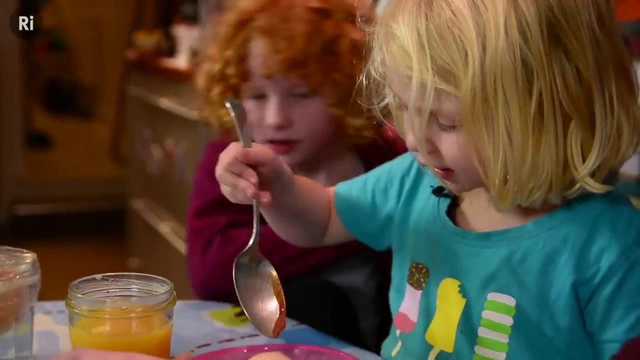 What do you think is going to happen? I'm going to get it out. I'm interested to see what's happened to our egg. Oh, look at all of those bubbles. I really think you should feel that Squishy. The acid in the vinegar reacts with the egg shell, which is mostly formed of calcium carbonate.